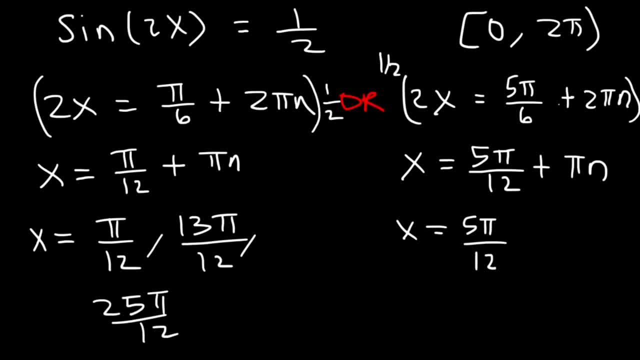 25 pi over 12 is more than 2 pi, because 2 pi is 24 pi over 12, so we can't include this answer. It's not in the range, So we're going to stop at 13 pi over 12.. 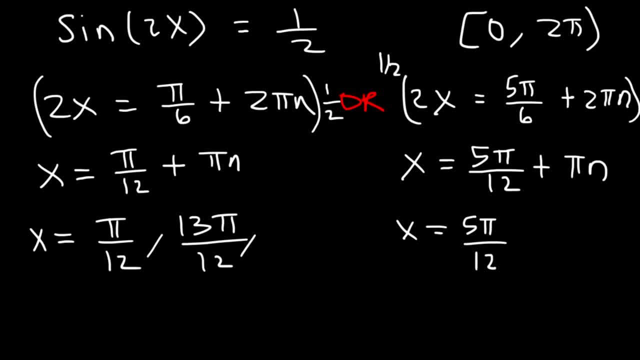 Now let's add pi n to 5 pi over 12.. So 5 pi over 12 plus 12 pi over 12, that's 17 pi over 12.. If we add pi n again, that would take us to 29 pi over 12,, which exceeds 2 pi. 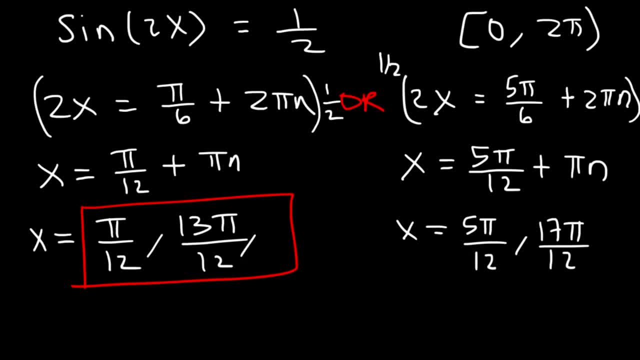 So we're going to stop here. These are the four answers. So notice that if this was simply x, we would have two answers: Pi over 6 and 5 pi over 6.. But since we have 2x, the number of answers in this range doubles. 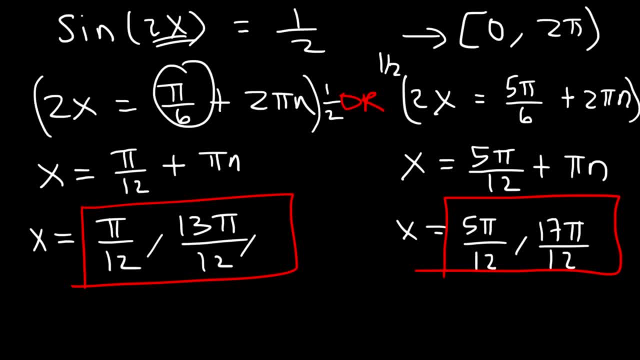 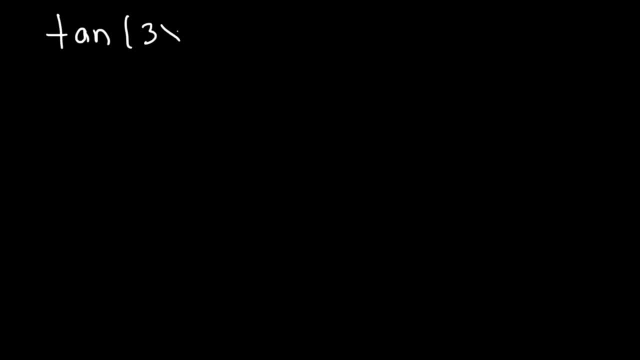 So instead of having two answers, we now have four answers. Let's try another example: Tangent 3x. Let's say it's equal to negative. 1. Find all solutions in the interval from 0 to 2 pi. Now we know that tangent of 45, or pi over 4, is positive 1.. 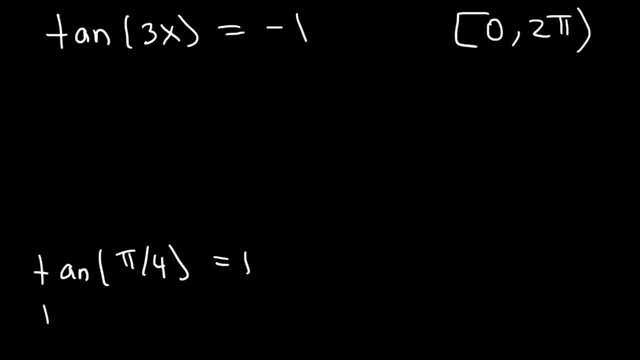 And tangent is negative in quadrants 2 and 4.. So tangent of 3 pi over 4 is negative, 1. And tangent of 7 pi over 4 is also negative, 1. So therefore we could say that 3x is equal to 3 pi over 4, plus pi n. 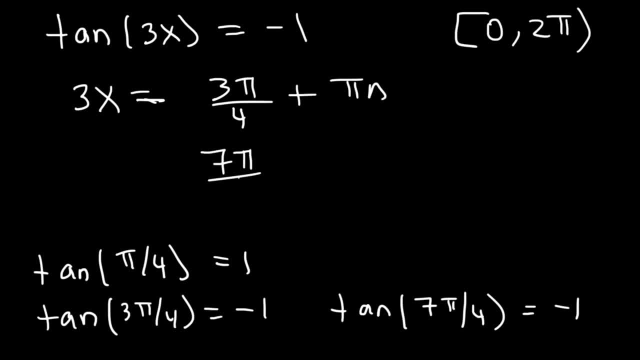 By the way, we don't have to say that it's equal to 7 pi over 4 plus pi n, Because pi n We'll give you this answer: When n is 1, you'll have 3 pi over 4 plus pi. 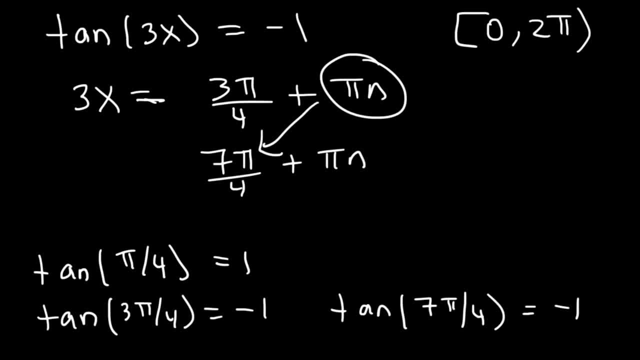 Pi is the same as 4 pi over 4.. So 3 pi over 4 plus 4 pi over 4 is 7 pi over 4.. So we can get all answers by simply making just this statement. Now let's multiply everything by 1. third, 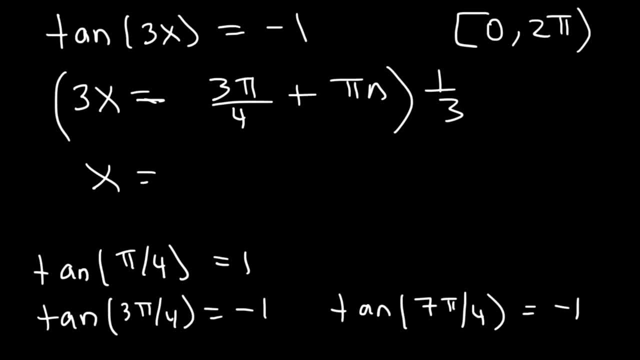 3x times 1. third or 3x divided by 3, is x 3 pi over 4 divided by 3. It's just pi over 4.. And then plus pi over 3 times n. So now let's get all answers in the range from 0 to 2 pi. 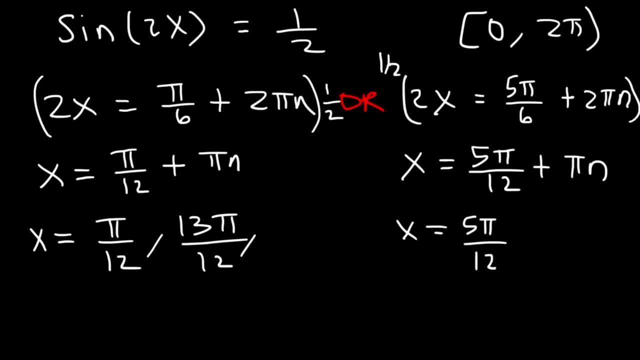 It's not in the range, So we're going to stop at 13 pi over 12.. Now let's add pi n to 5 pi over 12.. So 5 pi over 12 plus 12 pi over 12, that's 17 pi over 12.. 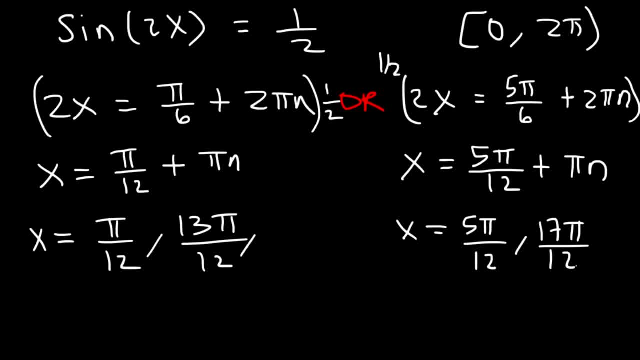 If we add pi n again, that would take us to 29 pi over 12,, which exceeds 2 pi. So we're going to stop here. These are the four answers. So notice that if this was simply x, we would have two answers. 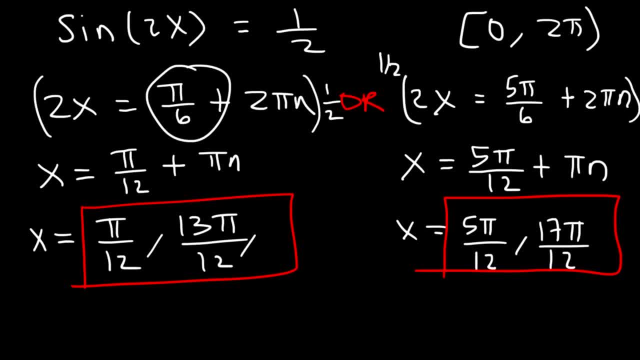 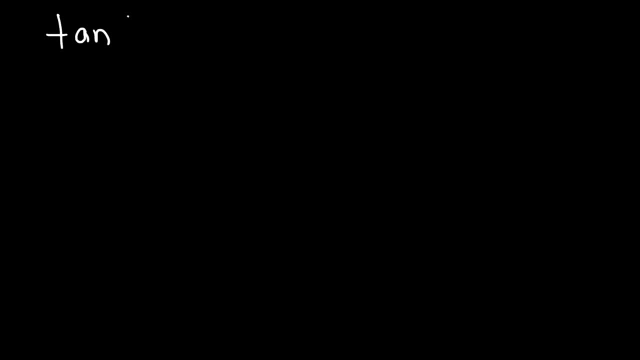 Pi over 6 and 5 pi over 6.. But since we have 2x, the number of answers in this range doubles. So instead of having two answers, we now have four answers. Let's try another example: Tangent 3x. 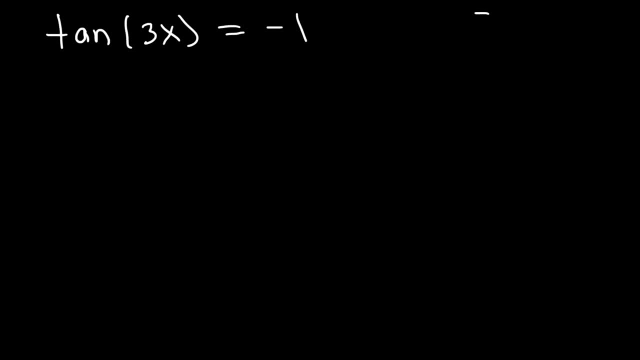 Let's say it's equal to negative. 1. Find all solutions in the interval from 0 to 2 pi. Now we know that tangent of 45, or pi over 4, is positive, 1. And tangent is negative in quadrants 2 and 4.. 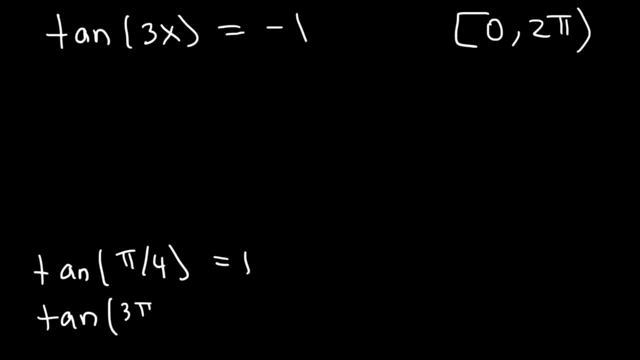 So tangent of 3 pi over 4 is negative 1. And tangent of 7 pi over 4 is also negative 1. So therefore we can say that 3x is equal to 3 pi over 4, plus pi n. 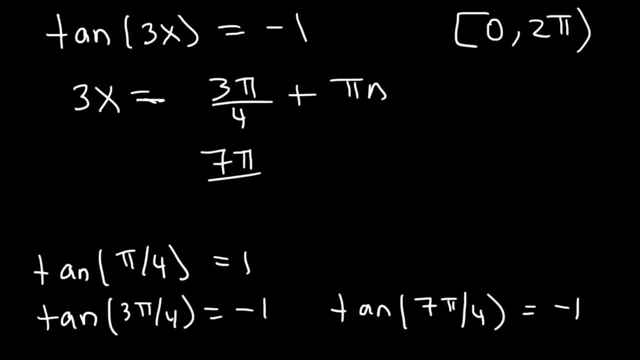 By the way, we don't have to say that it's equal to 7 pi over 4 plus pi n, Because pi n We'll give you this answer: When n is 1, you'll have 3 pi over 4 plus pi. 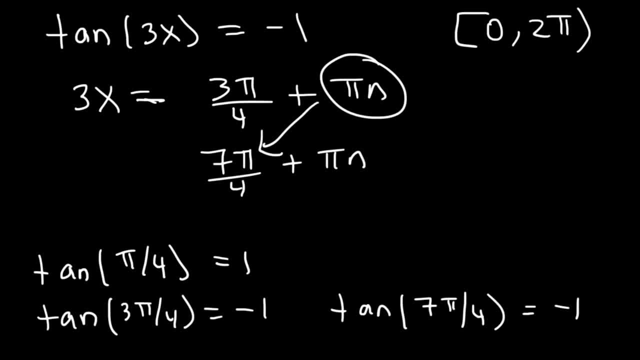 Pi is the same as 4 pi over 4.. So 3 pi over 4 plus 4 pi over 4 is 7 pi over 4.. So we can get all answers by simply making just this statement. Now let's multiply everything by 1. third, 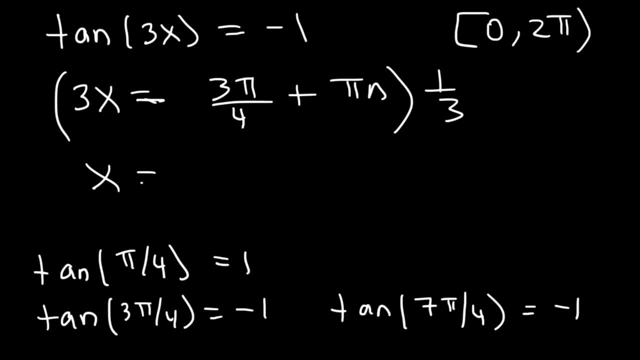 3x times 1. third or 3x divided by 3, is x 3 pi over 4 divided by 3. It's just pi over 4.. And then plus pi over 3 times n. So now let's get all answers in the range from 0 to 2 pi. 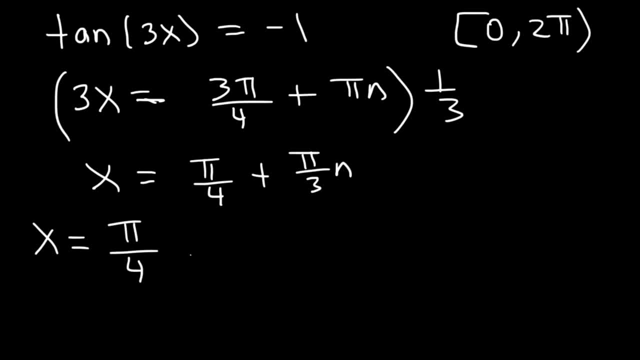 So when n is 0, the first answer is pi over 4.. Now, what about when n is 1?? So we're going to have- Let's make some space- When n is 1, we're going to have pi over 4.. 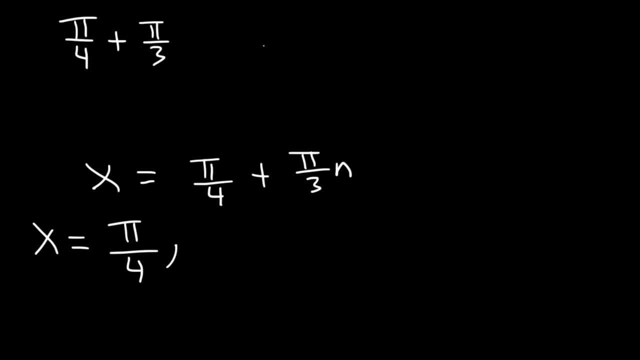 Plus pi over 3. So we need to get common denominators. So pi over 4, we need to multiply that by 3. So that becomes 3, pi over 12. And pi over 3, we've got to multiply that by 4 over 4.. 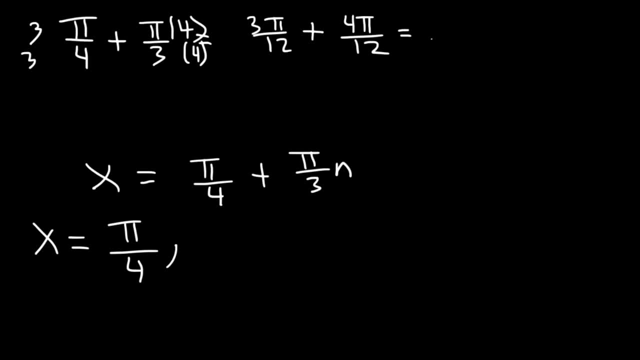 So that's plus 4 pi over 12.. Which becomes 7 pi over 12.. So that's the next answer. I'm going to rewrite this equation in terms of 12.. So this equation is 3 pi over 12 plus 4 pi over 12 times n. 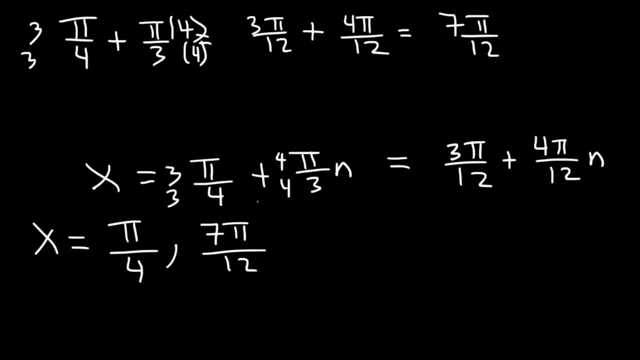 I just multiply this by 3 over 3 and this one by 4 over 4.. So I don't have to keep getting common denominators. So I'm going to use this equation to get the other answers. Now, what about when n is 2?? 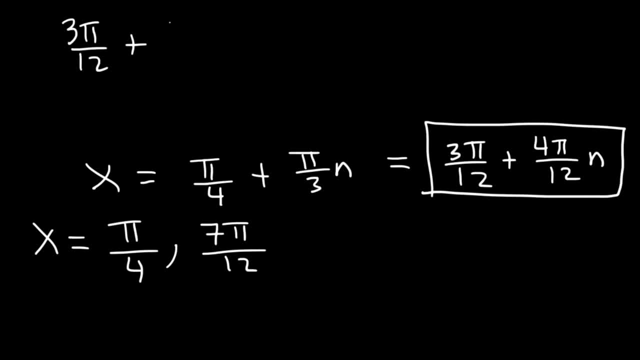 So this is going to be 3 pi over 12 plus 4 pi over 12 times 2. Which is 3 pi over 12 plus 8 pi over 12. And that's going to give us 11 pi over 12.. 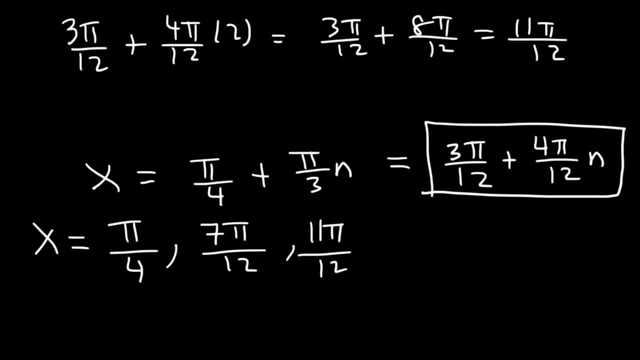 Notice that we're just going to keep adding 4 pi over 12.. I'm just going to write this as 3 pi over 12.. If we add 4 pi over 12 again, The next one is going to be 15 pi over 12.. 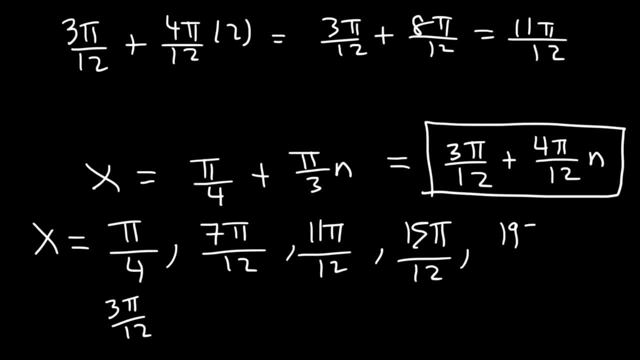 And then if we add another 4 pi over 12. It's going to be 19 pi over 12.. And if we do it again, 19 plus 4, 23 pi over 12.. And so forth. Now we can reduce this answer. 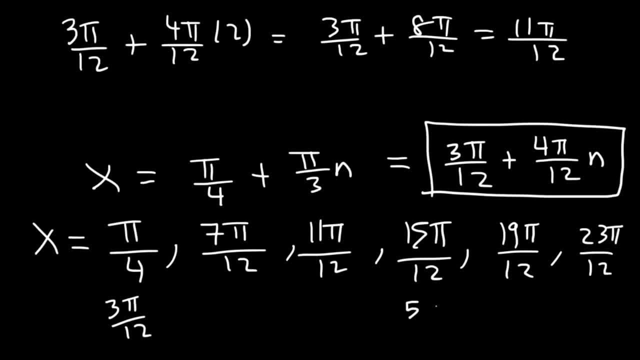 It's divisible by 3. So you can say that's 5 pi over 4. if you want Now, should we? Should we add 4 pi over 12 again to 23 pi over 12?? If we do, we'll get 27 pi over 12.. 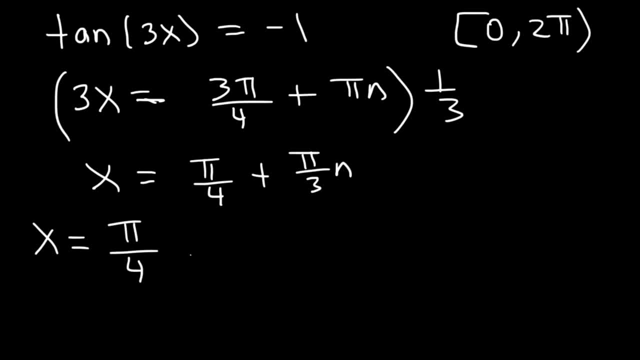 So when n is 0, the first answer is pi over 4.. Now, what about when n is 1?? So we're going to have- Let's make some space- When n is 1, we're going to have pi over 4.. 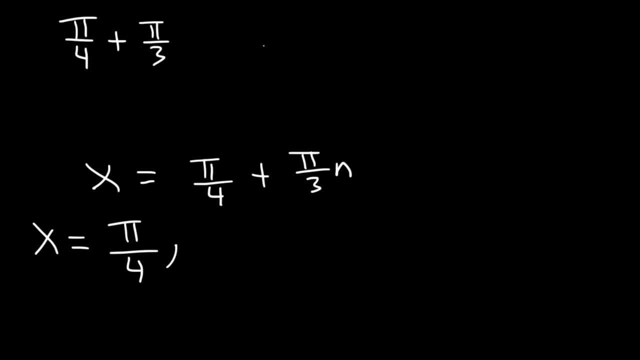 Plus pi over 3. So we need to get common denominators. So pi over 4, we need to multiply that by 3. So that becomes 3, pi over 12. And pi over 3, we've got to multiply that by 4 over 4.. 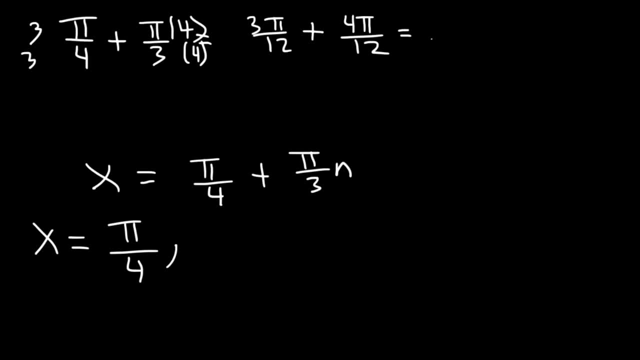 So that's plus 4 pi over 12.. Which becomes 7 pi over 12.. So that's the next answer. I'm going to rewrite this equation in terms of 12.. So this equation is 3 pi over 12 plus 4 pi over 12 times n. 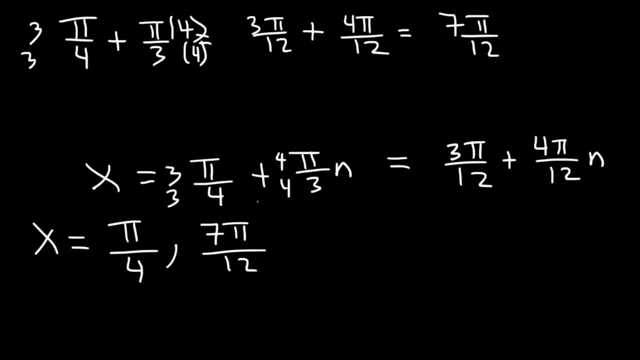 I just multiply this by 3 over 3 and this one by 4 over 4.. So I don't have to keep getting common denominators. So I'm going to use this equation to get the other answers. Now, what about when n is 2?? 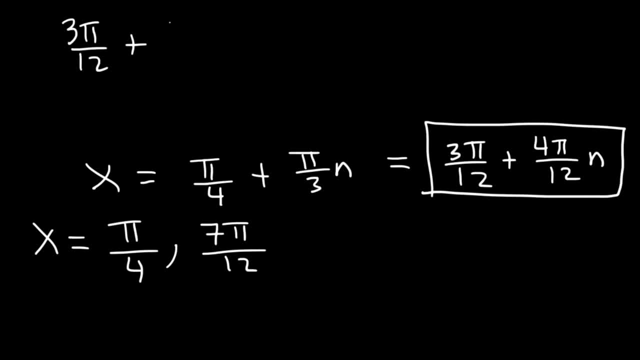 So this is going to be 3 pi over 12 plus 4 pi over 12 times 2. Which is 3 pi over 12 plus 8 pi over 12. And that's going to give us 11 pi over 12.. 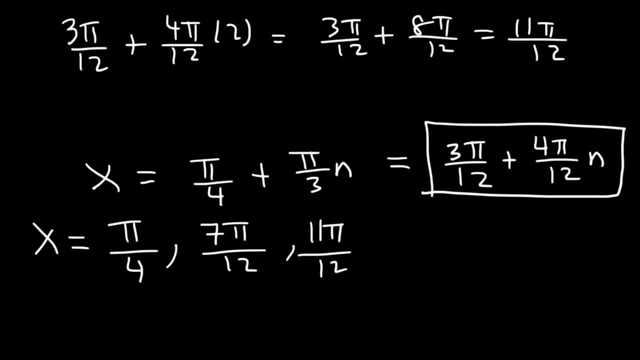 Notice that we're just going to keep adding 4 pi over 12.. I'm just going to write this as 3 pi over 12.. If we add 4 pi over 12 again, The next one is going to be 15 pi over 12.. 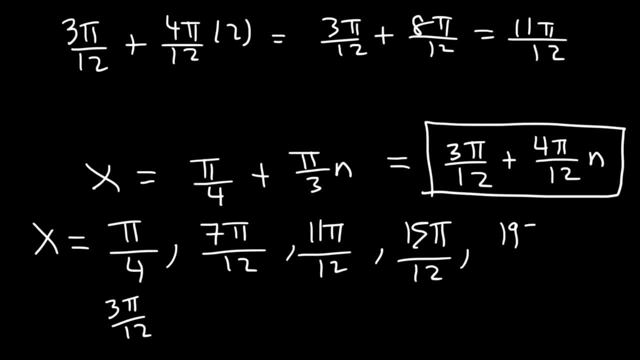 And then if we add another 4 pi over 12. It's going to be 19 pi over 12.. And if we do it again, 19 plus 4, 23 pi over 12.. And so forth. Now we can reduce this answer. 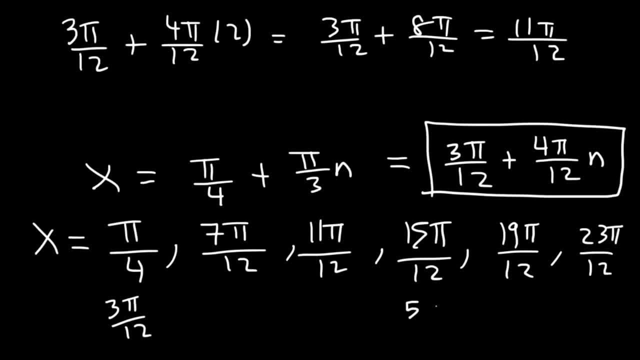 It's divisible by 3. So you can say that's 5 pi over 4. if you want Now, should we? Should we add 4 pi over 12 again to 23 pi over 12?? If we do, we'll get 27 pi over 12.. 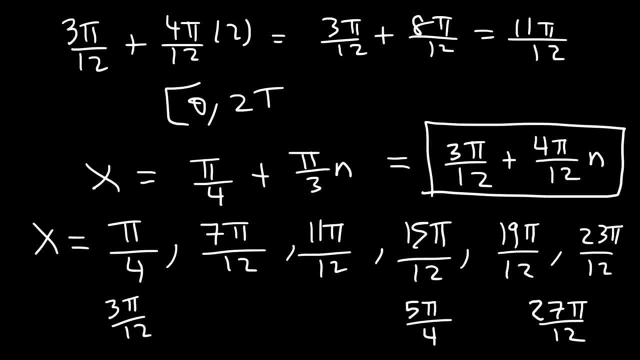 Now that answer isn't in the range of 0 to 2 pi. 12 times 2 is 24.. So if it exceeds 24 pi over 12, it's no longer in this range. So therefore we don't want this answer. 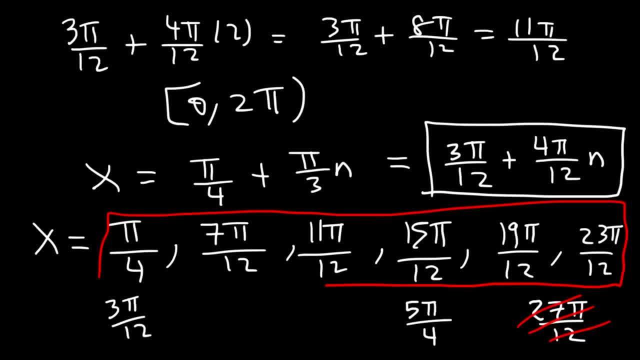 We're going to stop at 23 pi over 12.. Now let's say, if we have this equation, Tangent x is equal to negative 1.. There will only be 2 answers in this range, In quadrant 2 and quadrant 4.. 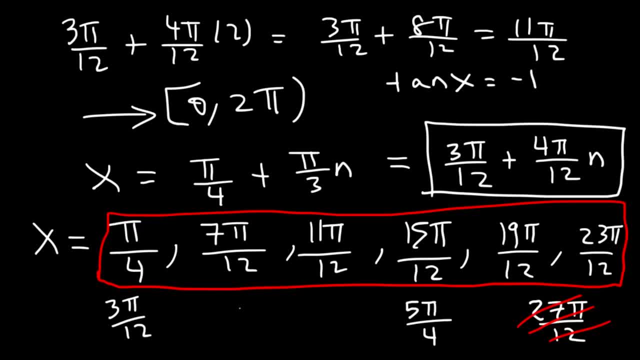 That would be 3 pi over 4 and 7 pi over 4.. But now, since we have a tan 3x expression, The number of answers triples from 2 to 6. So that can tell you when you should stop. 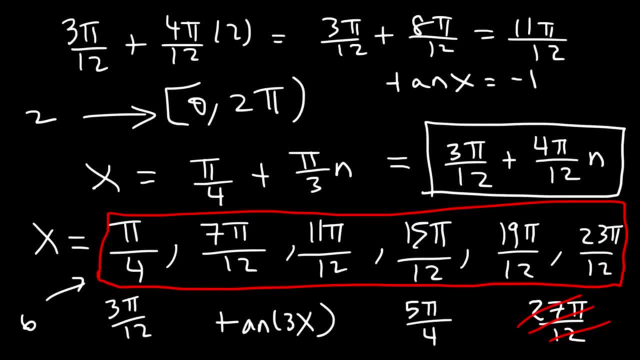 So if tangent x produces 2 answers, tangent 2x should give you 4 answers in this range. Tangent 3x should give you 6 answers in that range. Tangent 4x will give you 8.. Now, what about this one? 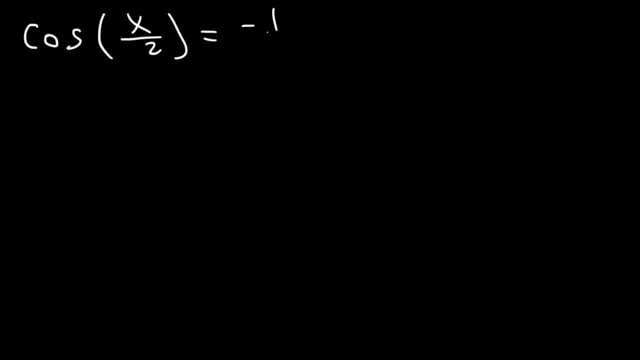 Cosine x divided by 2.. How many answers will exist in 0 to 2 pi? Now, if we had cosine x and if it was equal to negative 1 half, it would give you 2 answers. Cosine is negative in quadrants 2 and 3.. 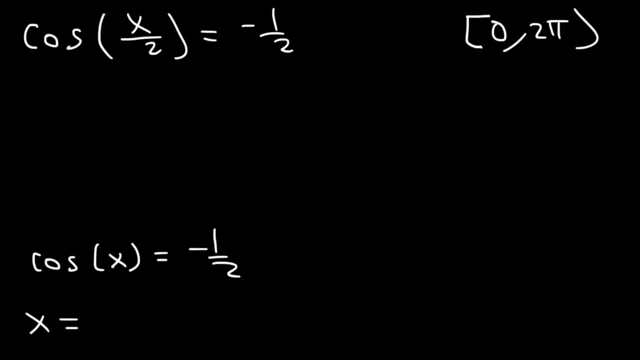 And so those 2 answers will be: They have a reference angle of 60 or pi over 3.. So they would be 2 pi over 3 and 4 pi over 3.. So with cosine x we'll get 2 answers in this range. 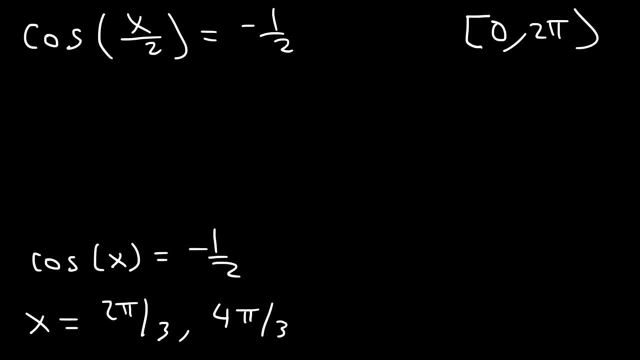 Cosine 2x will give us 4 answers. So cosine 1 half x should only give us 1 answer. So let's write this equation: This angle x over 2, has to be equal to 2 pi over 3 plus 2 pi n. 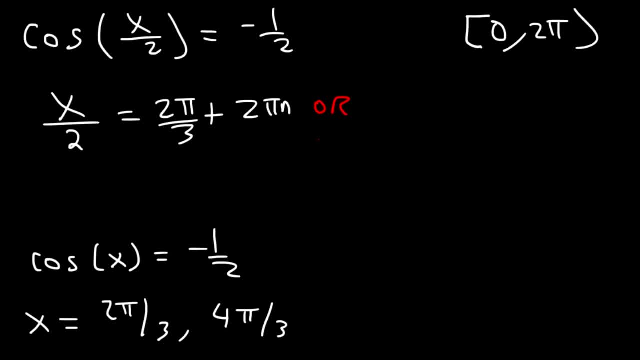 Or it could equal the other answer, That is, 4 pi over 3 plus 2 pi n. So let's multiply this answer by 2. to isolate x 2 times x over 2 is x 2 times 4 pi over 3.. 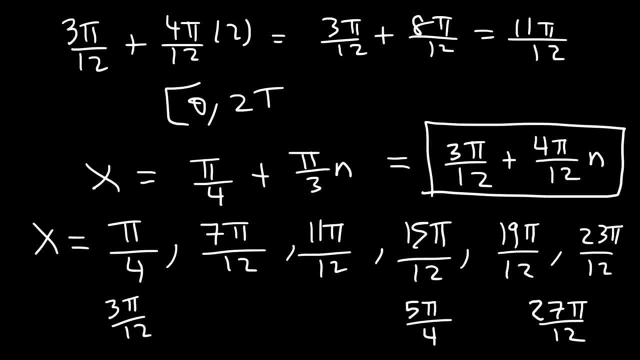 Now that answer isn't in the range of 0 to 2 pi. 12 times 2 is 24.. So if it exceeds 24 pi over 12, it's no longer in this range. So therefore we don't want this answer. 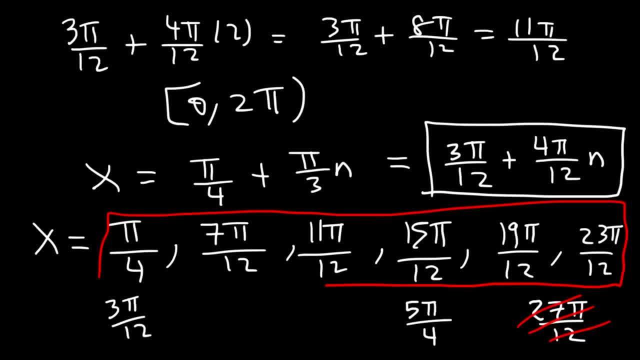 We're going to stop at 23 pi over 12.. Now let's say, if we have this equation, Tangent x is equal to negative 1.. There will only be 2 answers in this range, In quadrant 2 and quadrant 4.. 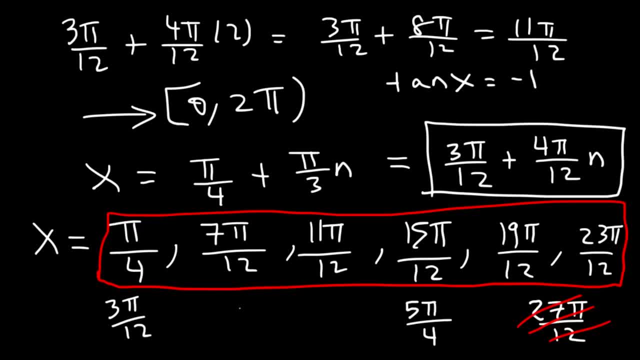 That would be 3 pi over 4 and 7 pi over 4.. But now, since we have a tan 3x expression, The number of answers triples from 2 to 6. So that can tell you when you should stop. 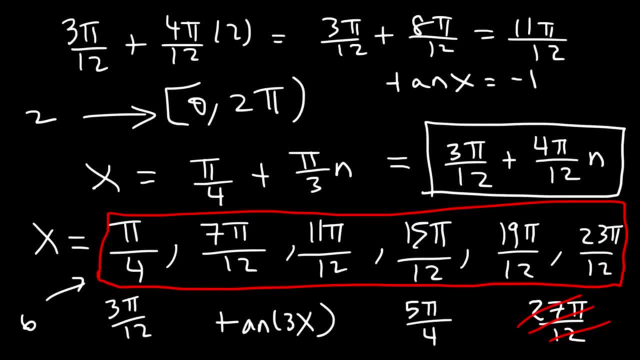 So if tangent x produces 2 answers, tangent 2x should give you 4 answers in this range. Tangent 3x should give you 6 answers in that range. Tangent 4x will give you 8.. Now, what about this one? 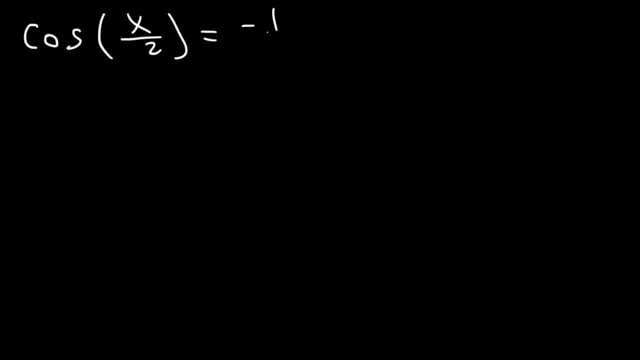 Cosine x divided by 2.. How many answers will exist in 0 to 2 pi? Now, if we had cosine x and if it was equal to negative 1 half, it would give you 2 answers. Cosine is negative in quadrants 2 and 3.. 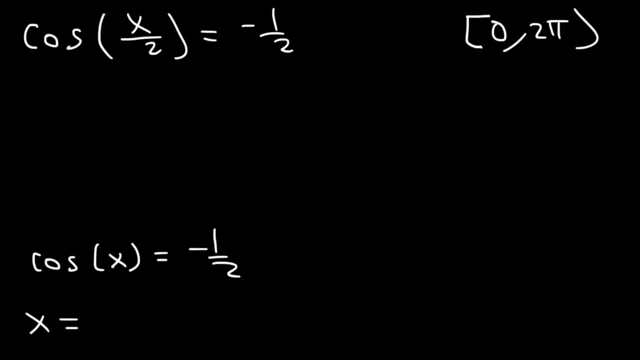 And so those 2 answers will be: They have a reference angle of 60 or pi over 3.. So they would be 2 pi over 3 and 4 pi over 3.. So with cosine x we'll get 2 answers in this range. 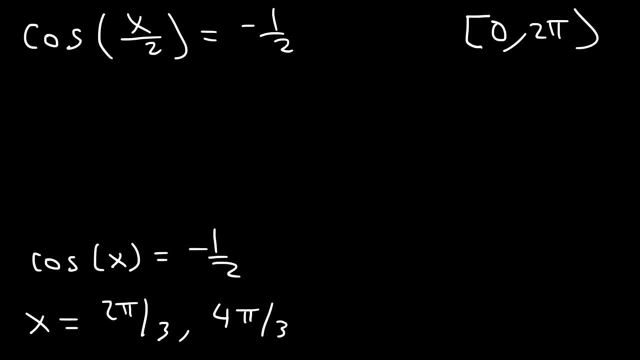 Cosine 2x will give us 4 answers. So cosine 1 half x should only give us 1 answer. So let's write this equation: This angle x over 2, has to be equal to 2 pi over 3 plus 2 pi n. 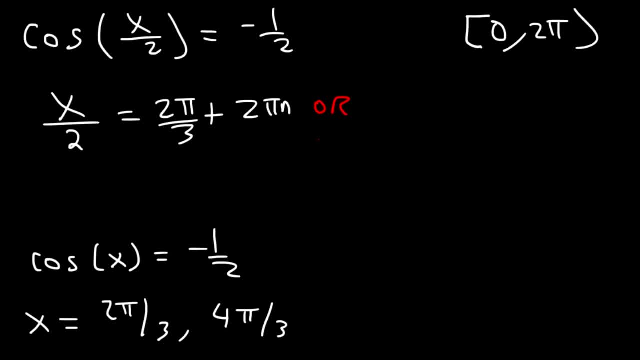 Or it could equal the other answer, That is, 4 pi over 3 plus 2 pi n. So let's multiply this answer by 2. to isolate x 2 times x over 2 is x 2 times 4 pi over 3.. 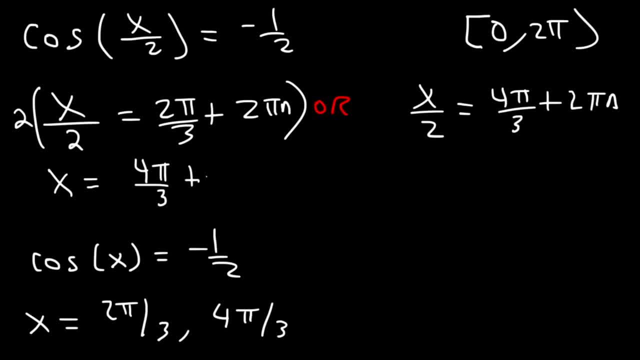 I mean 2 times 2 pi over 3 is 4 pi over 3.. And then plus 4 pi n. And here, if we multiply that by 2, we'll get x is equal to 8 pi over 3, plus 2 pi n. 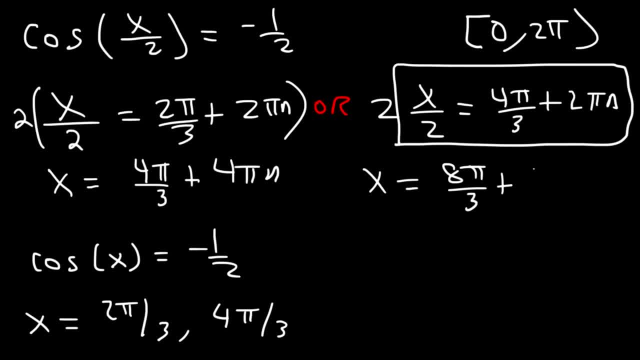 That should be 4 pi n, Not 2 pi n. Now, when n is 0,, what answers will we get? So using this equation? when n is 0,, the first answer is 4 pi over 3.. 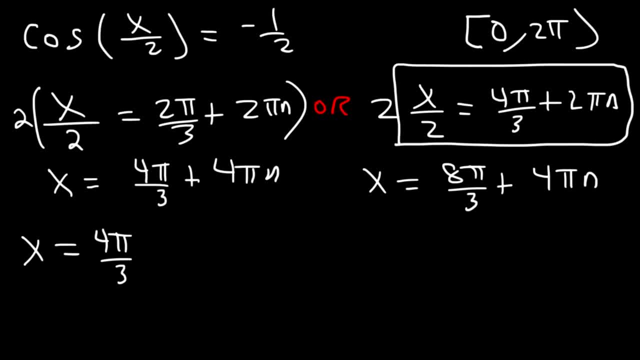 When n is 1,, 4 pi plus 4 pi over 3 will be much bigger than 2 pi, So that's not going to work. Let's try when n is negative: 1.. 4 pi over 3 minus 4 pi, which is like minus 12 pi over 3,. 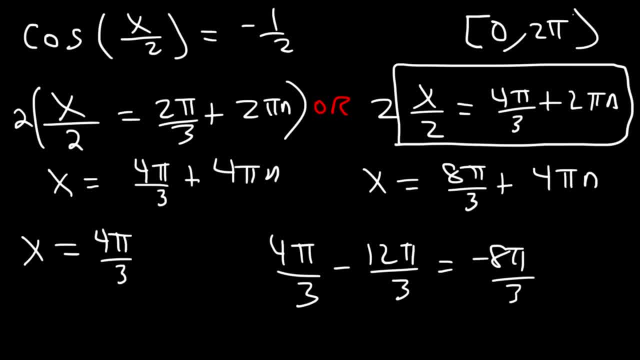 that's negative, 8 pi over 3, which is not in this range because only positive answers exist in that range. So in the first equation the only possible answer is simply 4 pi over 3.. There's no other answer that exists in the range. 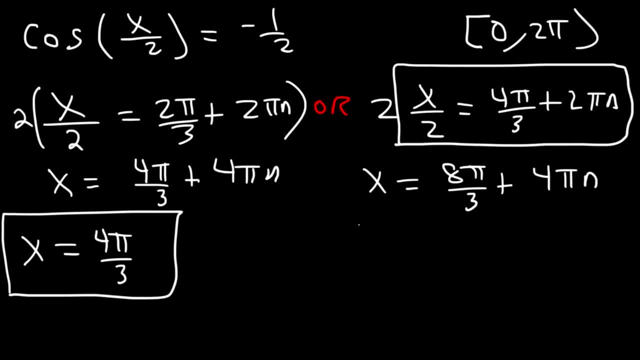 If we add or subtract by 4 pi, it's too much. Now, looking at this one, 8 pi over 3 already exceeds 2 pi. 6 pi over 3 is 2 pi, so 8 pi over 3 is greater than that. 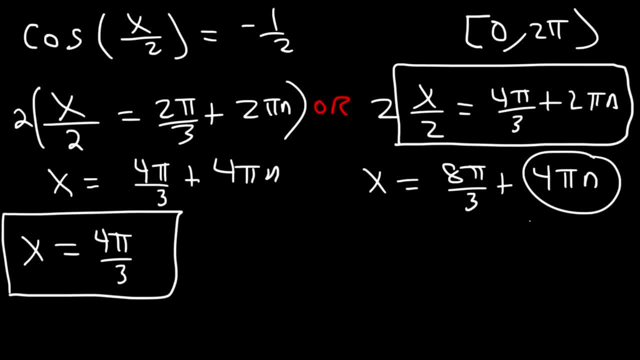 So that can't work. If we add 4 pi, it's going to be even larger. But what if we subtract by 4 pi? So 4 pi is 12 pi over 3, and this would give us negative 4 pi over 3.. 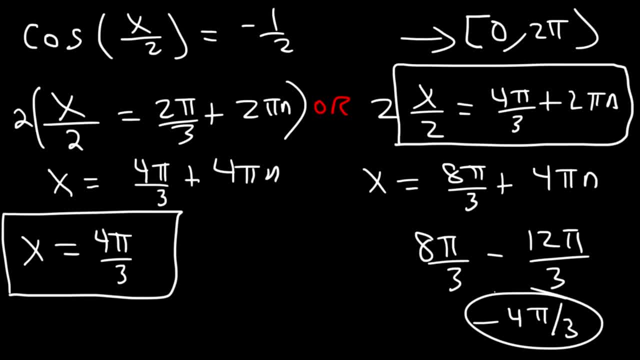 But it's still a negative answer and it's not in this range. So therefore, this is not going to give us any answer in the range of 0 to 2 pi. So we only have one answer for this particular problem. 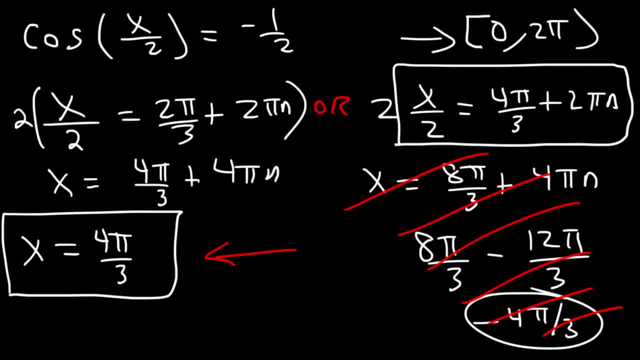 And it's just 4 pi over 3.. That's the only answer that will make this equation true and, at the same time, is within this range. So 1 half x only gave us one answer. 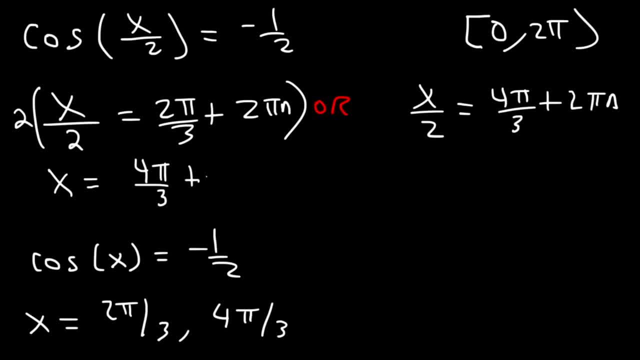 I mean 2 times 2 pi over 3 is 4 pi over 3.. And then plus 4 pi n. And here, if we multiply that by 2, we'll get x is equal to 8 pi over 3, plus 2 pi n. 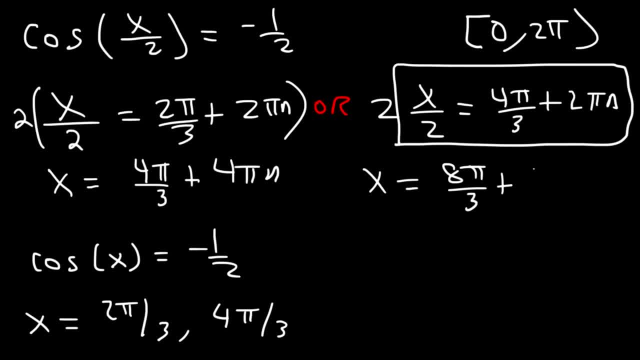 That should be 4 pi n, Not 2 pi n. Now, when n is 0,, what answers will we get? So using this equation? when n is 0,, the first answer is 4 pi over 3.. 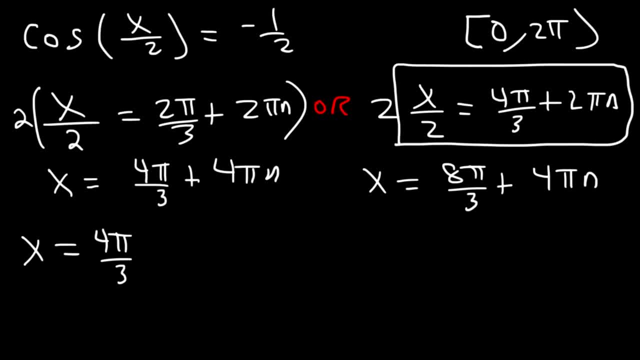 When n is 1,, 4 pi plus 4 pi over 3 will be much bigger than 2 pi, So that's not going to work. Let's try when n is negative: 1.. 4 pi over 3 minus 4 pi, which is like minus 12 pi over 3,. 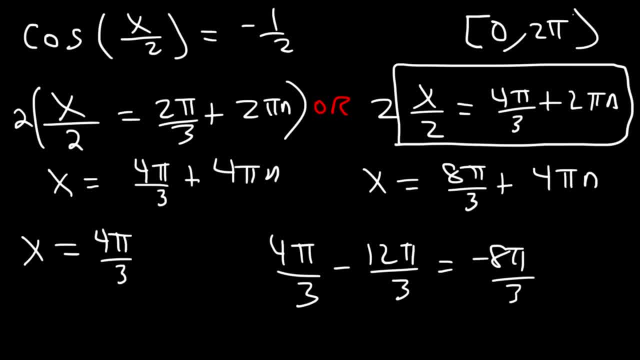 that's negative, 8 pi over 3, which is not in this range because only positive answers exist in that range. So in the first equation the only possible answer is simply 4 pi over 3.. There's no other answer that exists in the range. 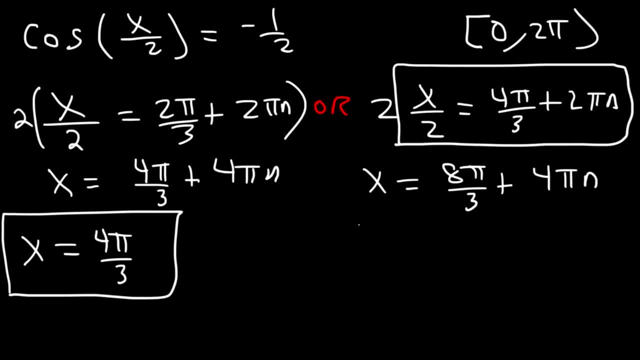 If we add or subtract by 4 pi, it's too much. Now, looking at this one, 8 pi over 3 already exceeds 2 pi. 6 pi over 3 is 2 pi, so 8 pi over 3 is greater than that. 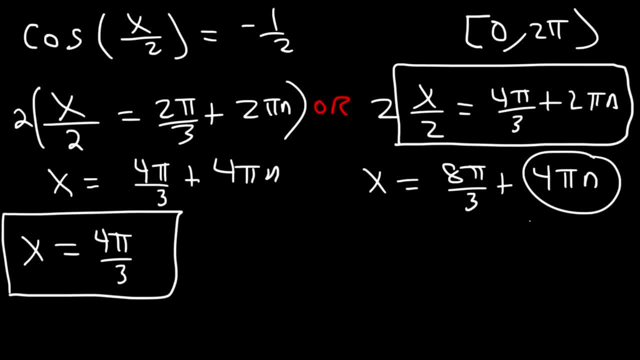 So that can't work. If we add 4 pi, it's going to be even larger. But what if we subtract by 4 pi? So 4 pi is 12 pi over 3, and this would give us negative 4 pi over 3.. 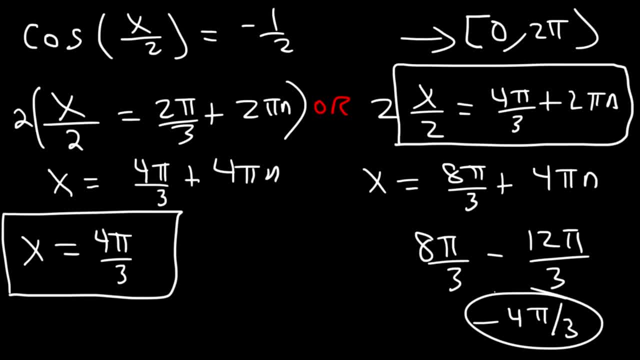 But it's still a negative answer and it's not in this range. So therefore, this is not going to give us any answer in the range of 0 to 2 pi. So we only have one answer for this particular problem. 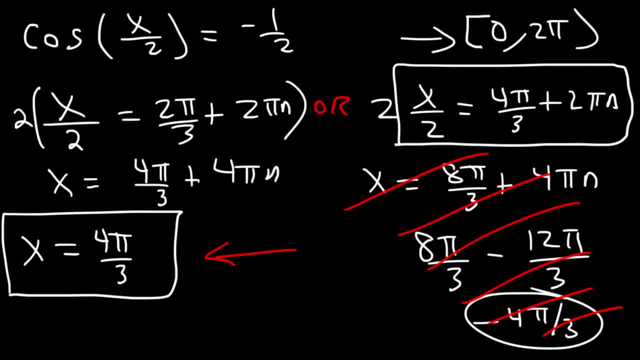 And it's just 4 pi over 3.. That's the only answer that will make this equation true and, at the same time, is within this range. So 1 half x only gives us one answer.